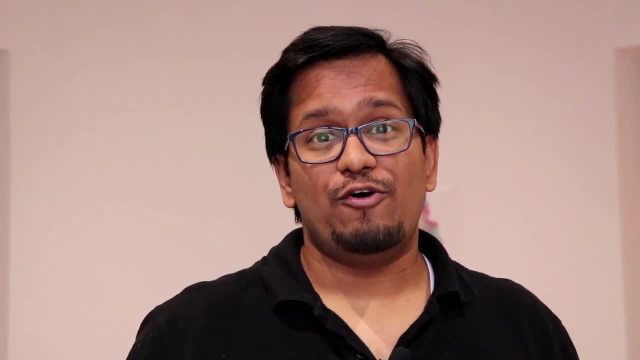 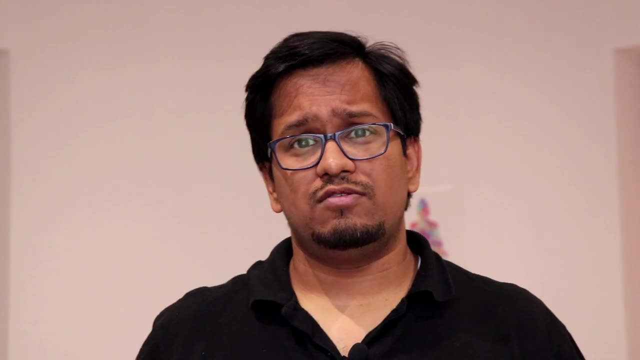 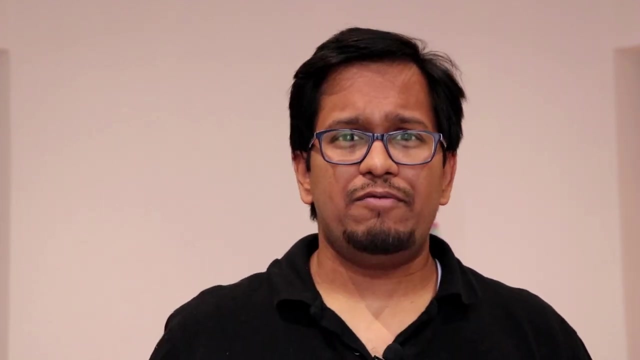 hello everyone. welcome back. as always, I hope you are doing absolutely fantastic in your life. so today in this video, we are going to talk about something called markup decision process. with markup decision process, we basically formalize sequential decision-making process. in our previous videos we didn't really 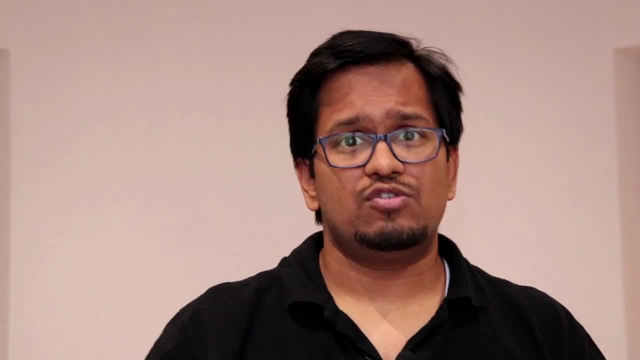 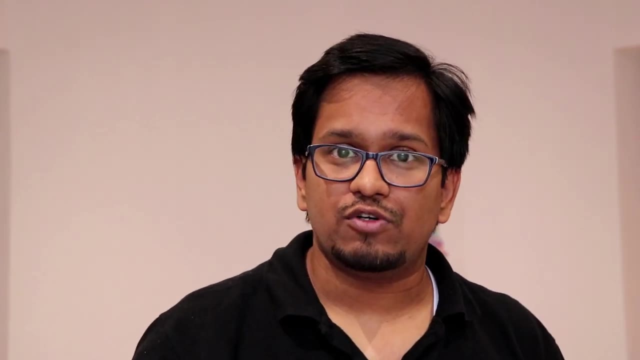 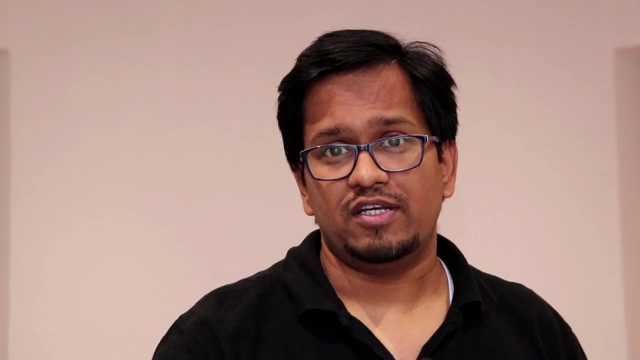 talk about how we formalize reinforcement learning. so in this video we focus on that. we formalize reinforcement learning. problem with mark of decision process. so what are the components of markup decision process? so there are five main components of Markov decision process in reinforcement learning. the number one is agent. the number two is the environment number. 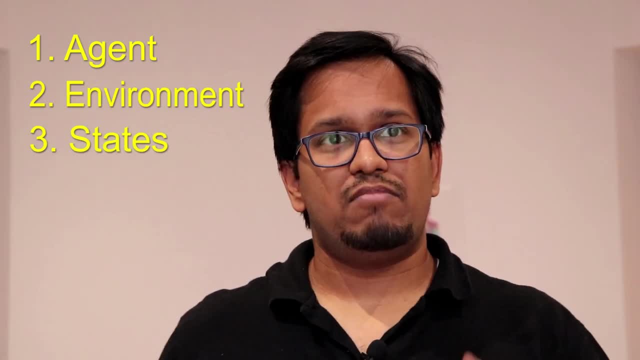 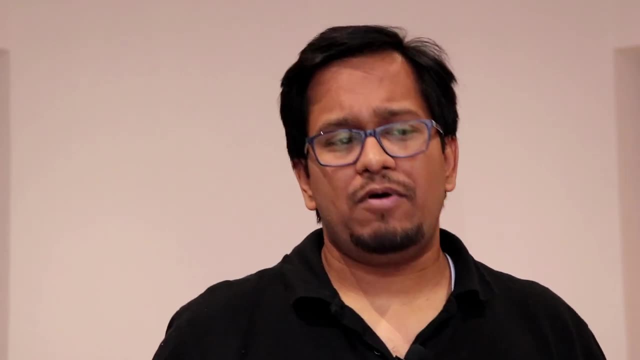 three, the improper state of the environment. Number four is the actions. Number 5: is심 are của� pastryю, 3.5% the reward. so there are five components. so let's talk about agent. so agent is the main decision maker in the reinforcement, learning or markup. 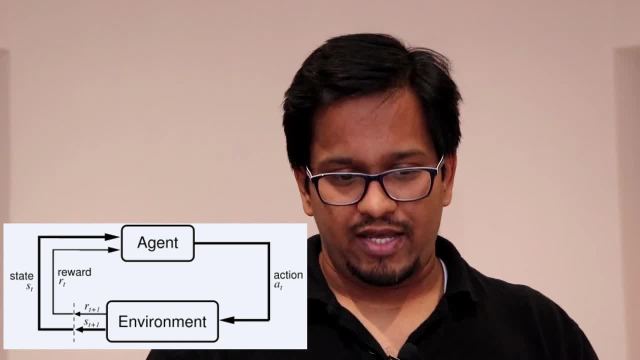 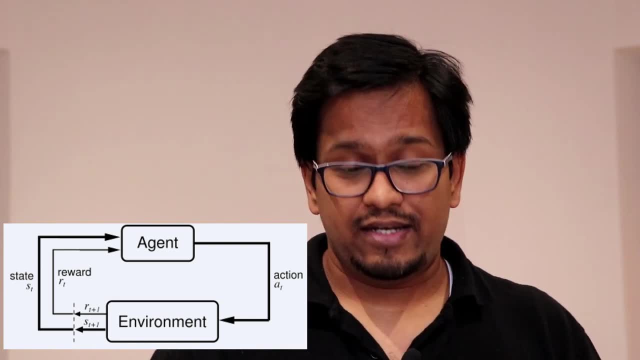 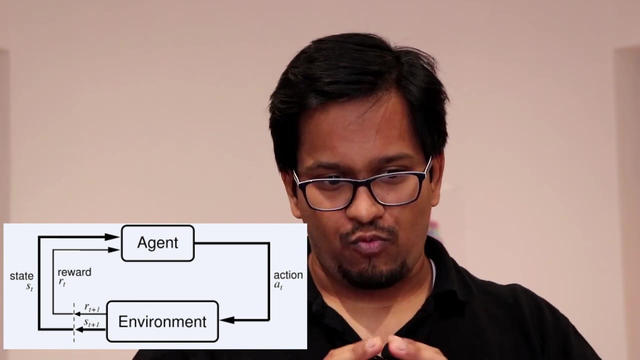 decision process. so it basically interacts with the environment. it takes, it takes an action in the environment, looking into the current state or current situation of the environment, and it applies that action and environment or the system moves to a different state. so, and going from one state by taking a, 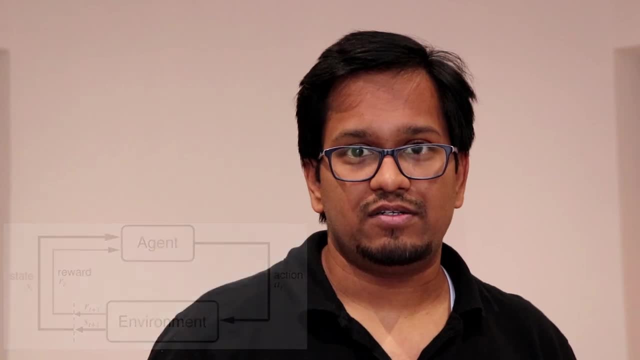 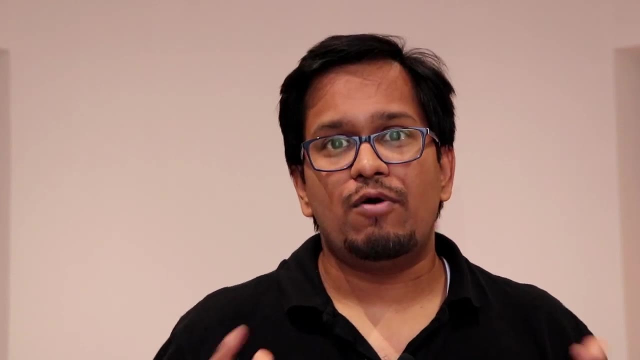 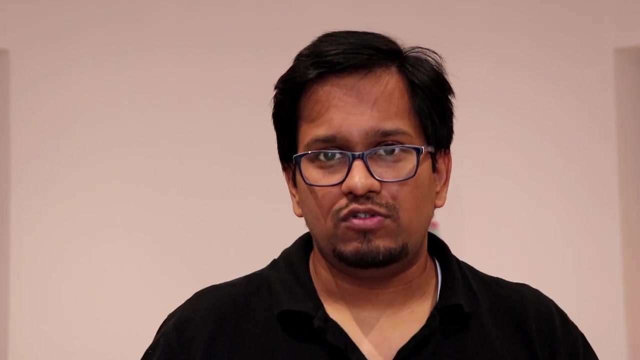 particular action. it gets some reward from the environment, so state basically defines the entire situation or it encodes the entire information of the state at the particular moment. so here we actually should talk about something called Markov property and we use this in reinforcement learning. so Markov- 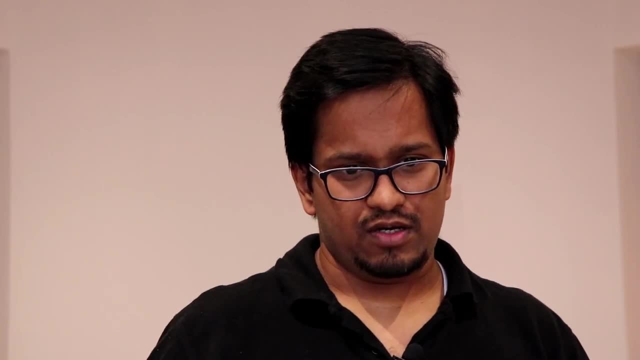 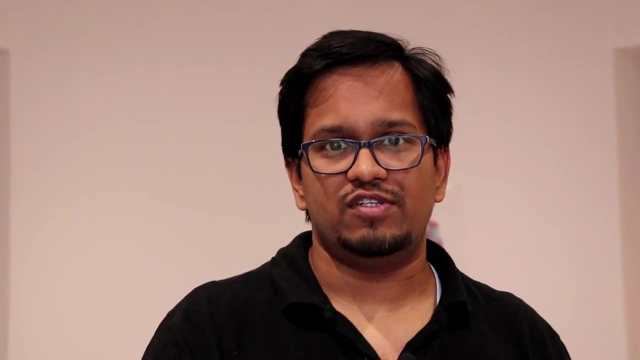 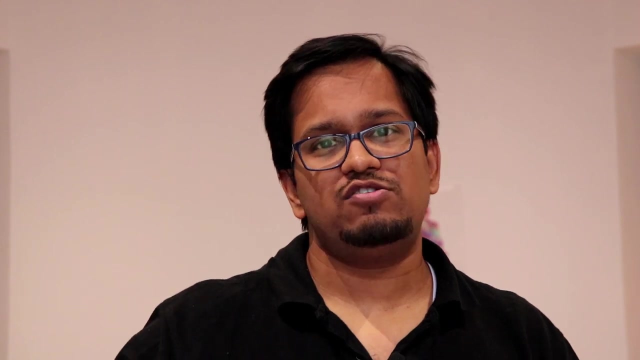 property is something related to the states. so when a system has Markov property associated with the states, then we can say that the state transition based on an action on the state depends only on the current state of the system and it doesn't depend on the entire state action reward. 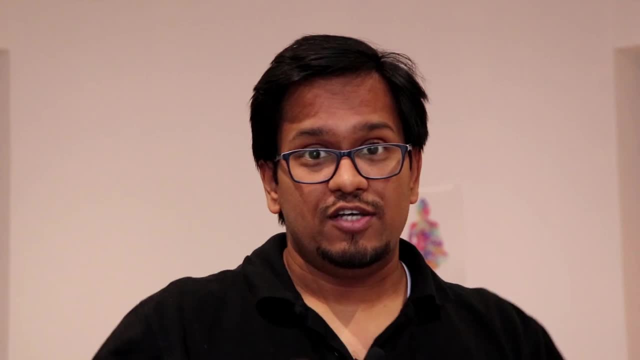 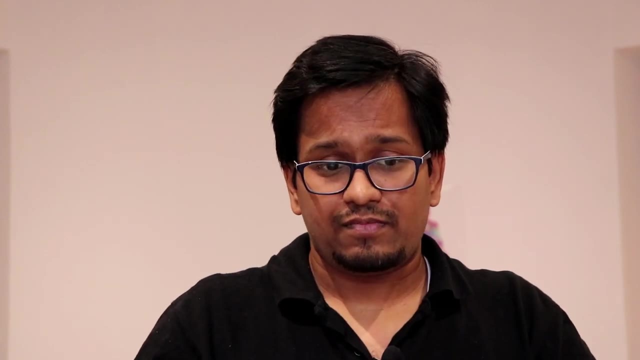 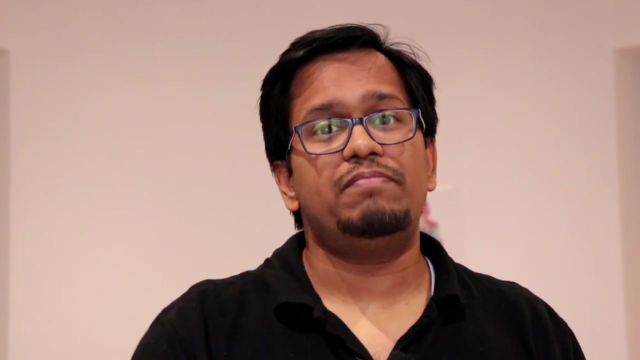 trajectory that happened in the past. are you getting my point? so if you are in a, if your agent in a particular state of the environment or state of the system, then if it takes an action, then the state transition, the the next state of the system, will depend only on the current state. 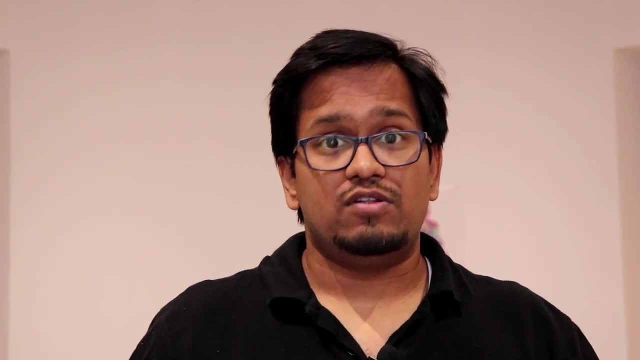 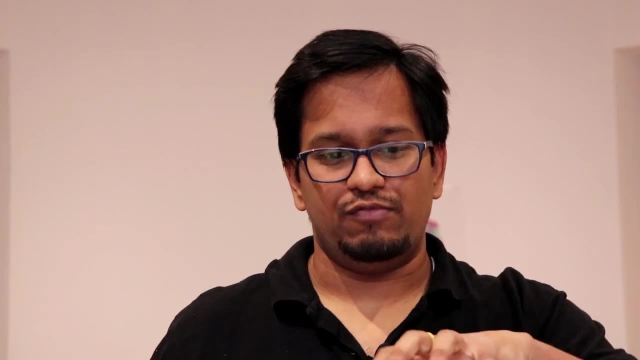 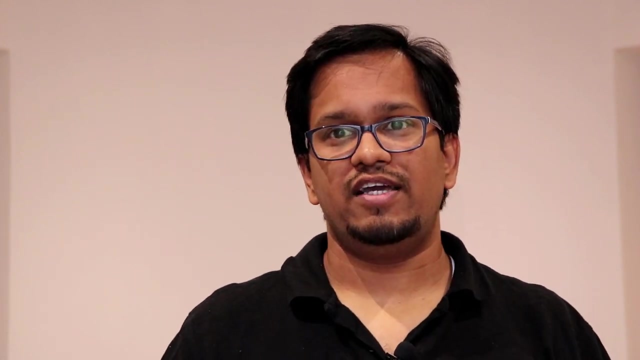 and current action of the environment. it will not depend on the previous actions and previous rewards or whatever happened in the past, so it will depend only on the present scenario. so this is the Markov property and we'll use it in reinforcement learning. now, when we talk about Markov decision process, we mainly 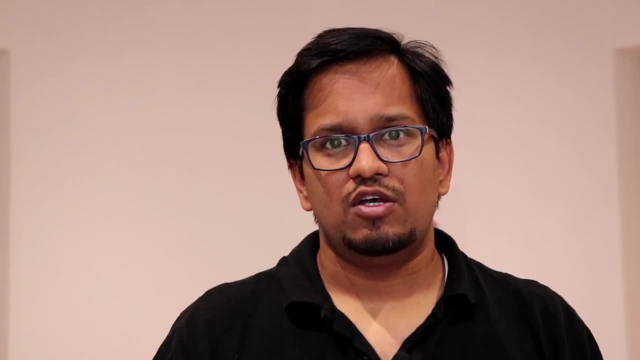 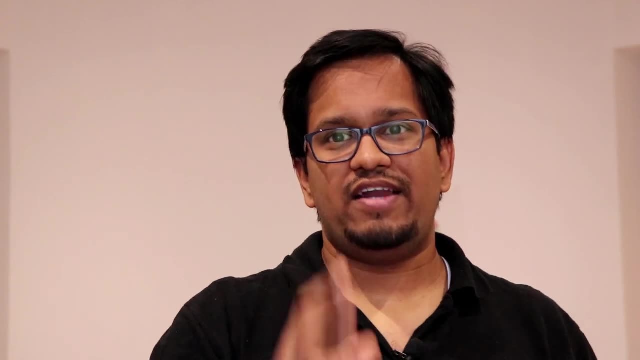 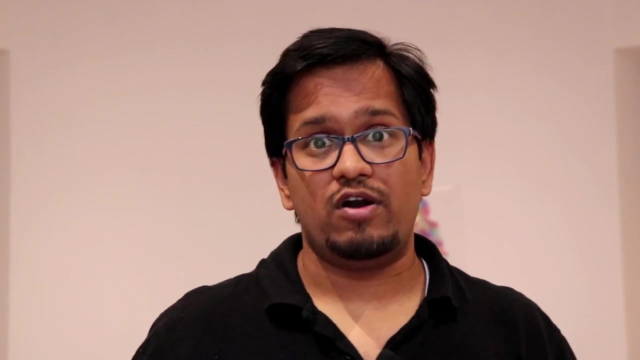 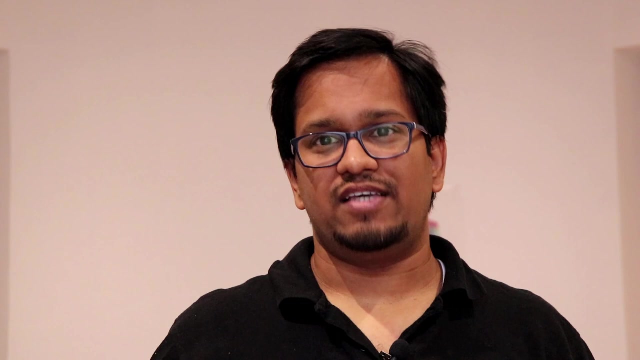 talk about finite Markov decision process. so in finite Markov decision process we assume that states are finite. so state has finite number of elements, the state set, the set of state has finite number of elements. set of reward has finite number of elements and state of action has finite number of elements. so let's take an example of chess game. so 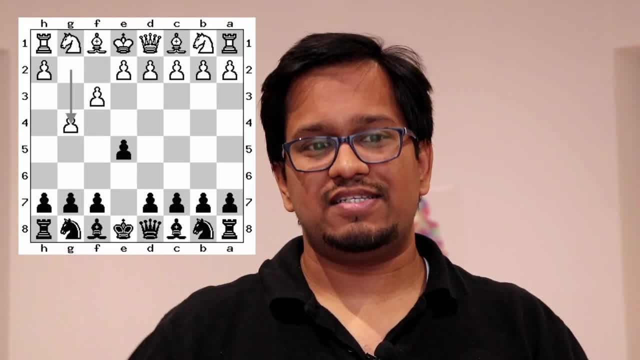 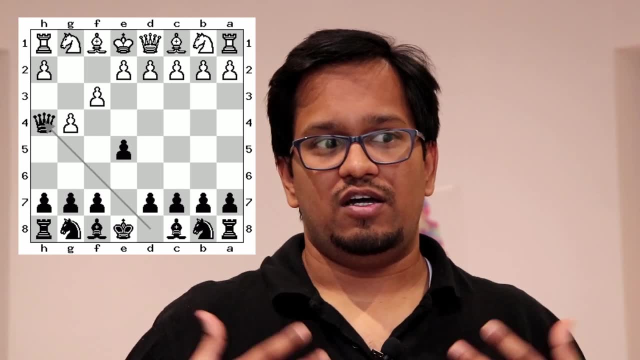 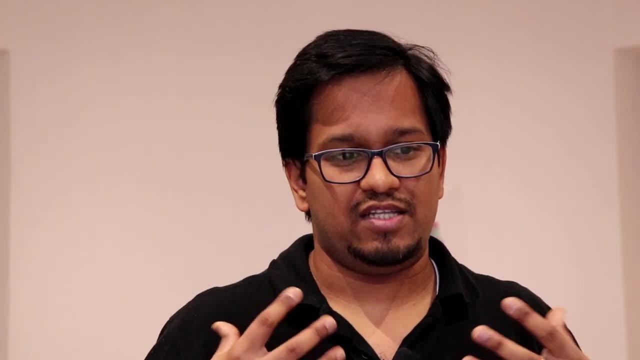 in chess game, the state- we define the state as the current position of the pieces of the chessboard. pieces means pawns, kings, queens, rooks, bishops, all the elements. and this state is actually Markovian if you think about it carefully, because if you're playing chess, you don't have to think about what. 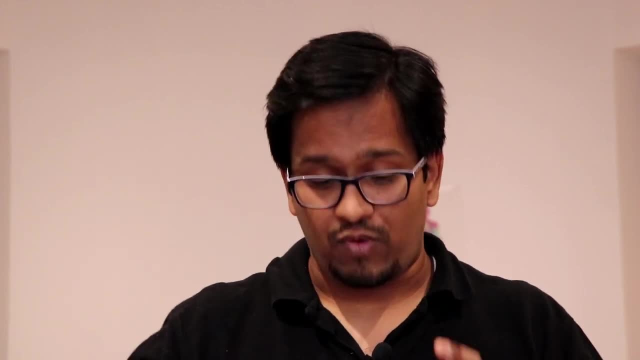 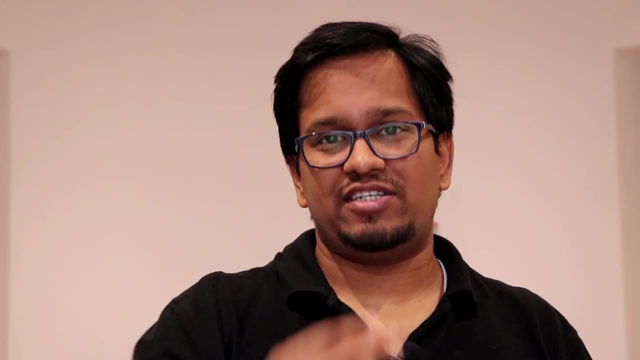 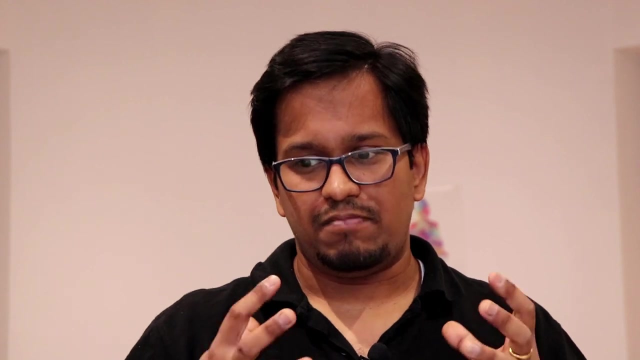 happened in the past. you just have to worry about what is the current situation of that state board- where are the pieces- and you can immediately take an action based on that current situation. you don't need to worry about what happened in the past. so this is Markovian if you see the same. 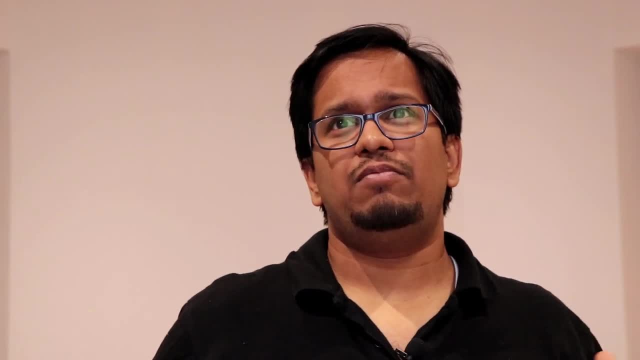 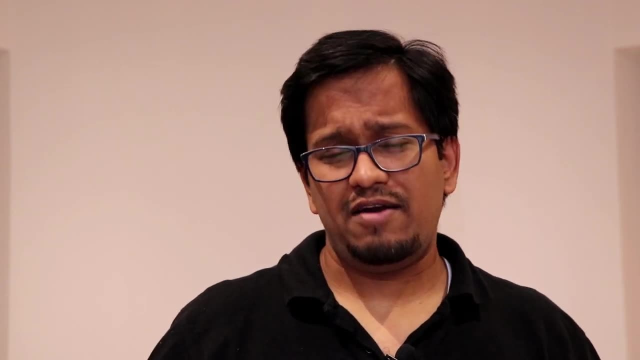 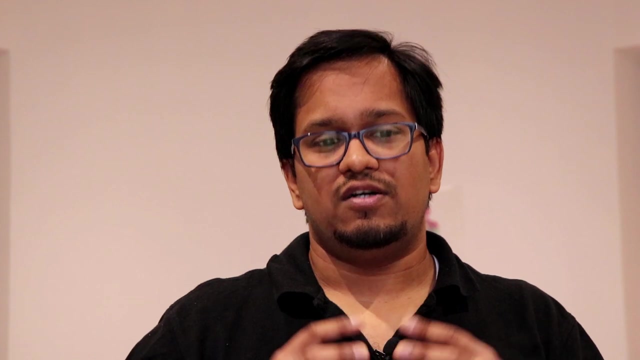 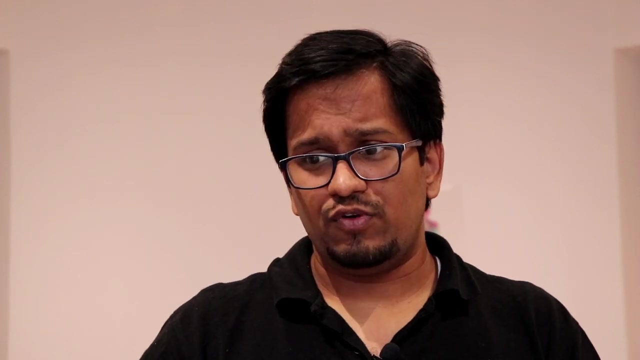 case of tic-tac-toe game. now let's take an example of something which is not Markovian. for example, if you talk about share market, so share market, if you see, you cannot exactly predict looking into the current state of the share market or particular share of a particular company. if you see what, if you think about what, 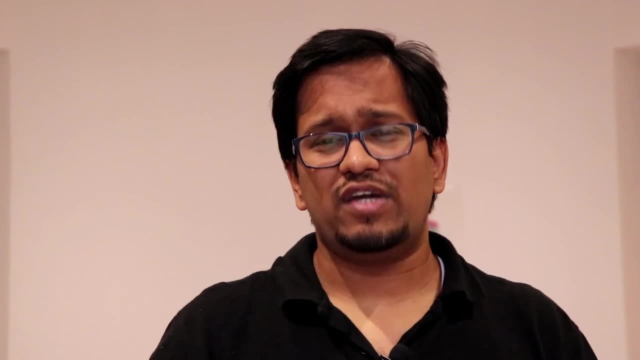 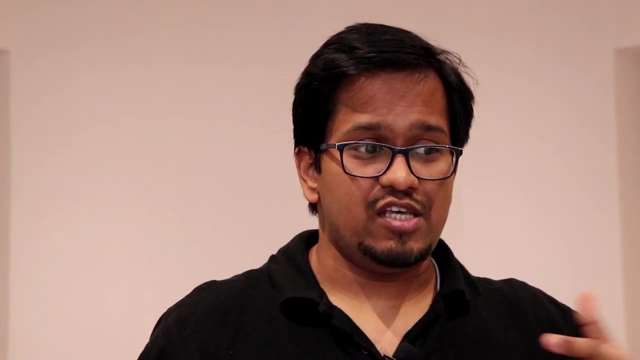 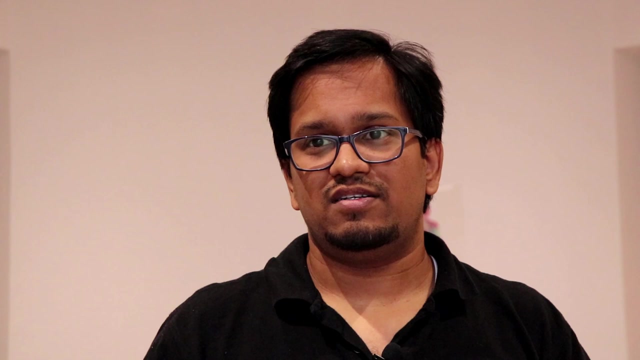 will be the share value. it will increase or decrease. you cannot really predict it looking into the today's information. you have to look into a sequence of events that happened in the past, so in that case you cannot actually take the optimal decision based on the current state. you need additional. 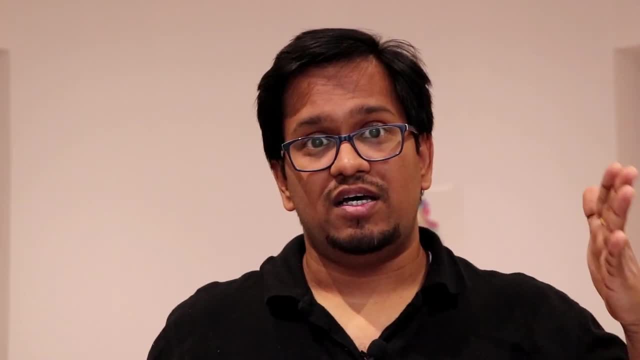 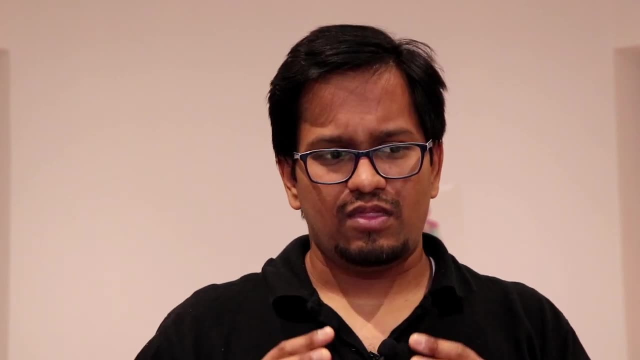 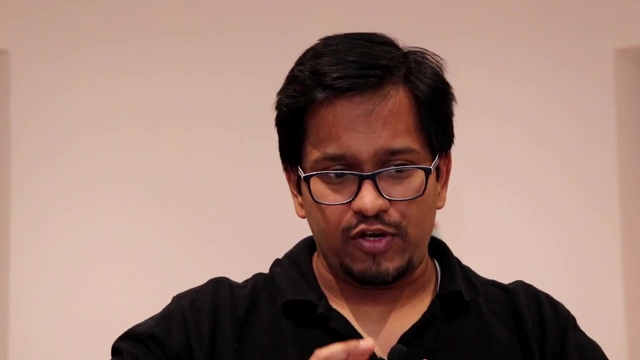 information, the sequence of events that happened in relation to that company. so this is this particular thing doesn't follow Markovian property and always remember Markovian property. Markov property is a property associated with the state. so if we define a state differently, then we 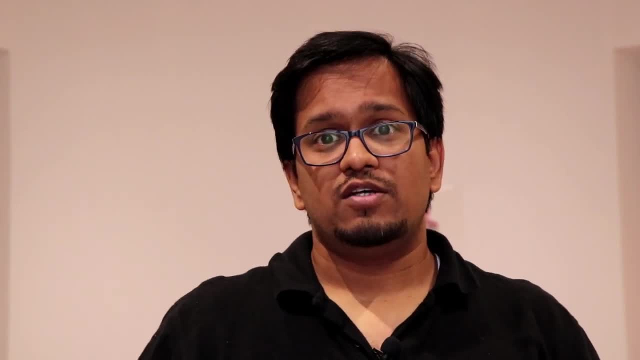 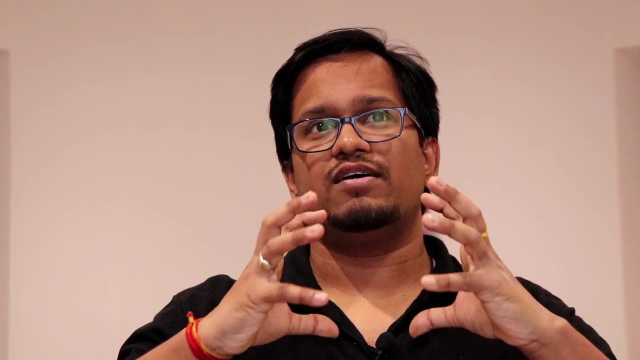 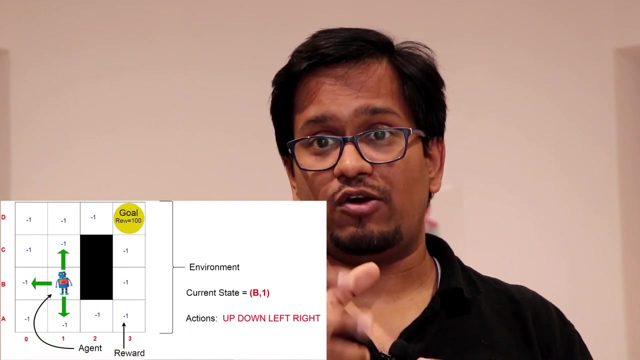 can make a system Markovian or non-Markovian. so this is, this is the way we define a reinforcement learning problem. so in reinforcement learning problem, what is the goal? the agent has to take action in the environment where the states are Markovian. that means it will just look into the current state of 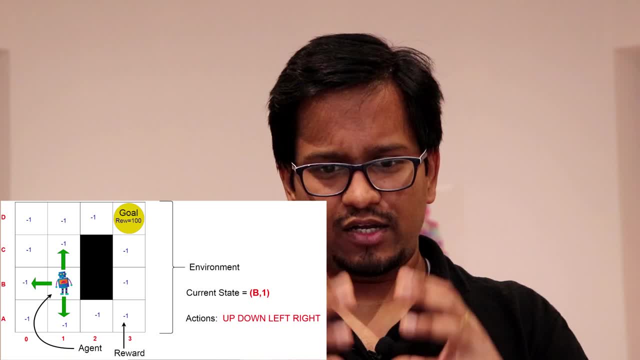 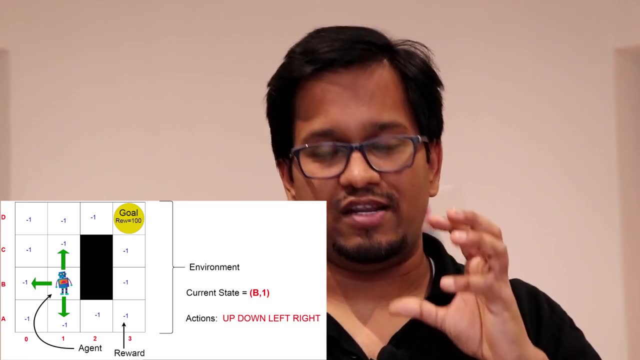 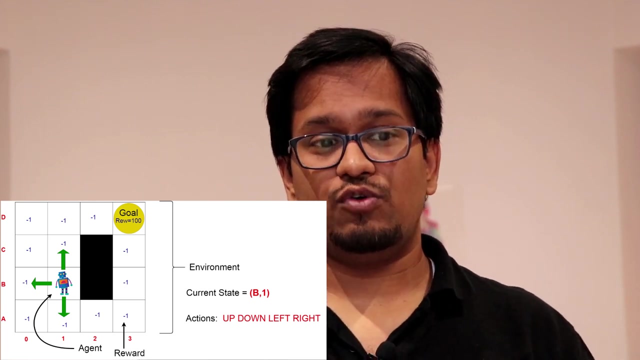 the system and it will take an action. and the goal of the agent is to increase the total reward in the system. so, since it gets a reward, once it applies an action at the particular state, it moves to a different state and during this transition it gets a reward, so it has to increase the total. 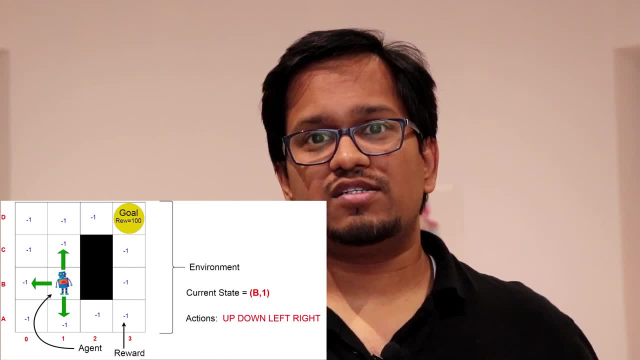 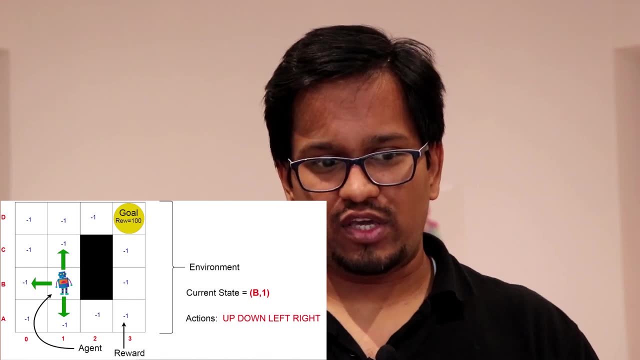 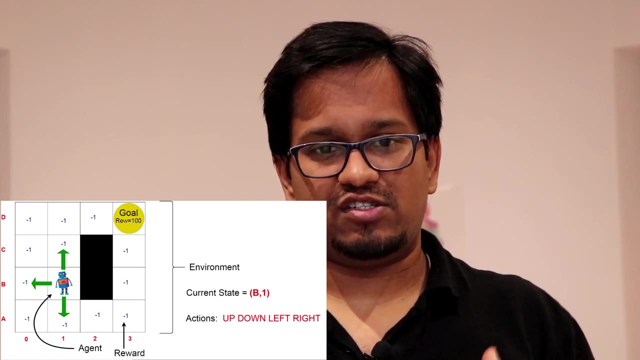 cumulative reward in the system. so it doesn't worry about what is the next reward, it doesn't care maximizing the next reward or immediate reward. it has to care about the total reward of the entire trajectory, the entire sequence of action, state action, reward sequence it has to worry about 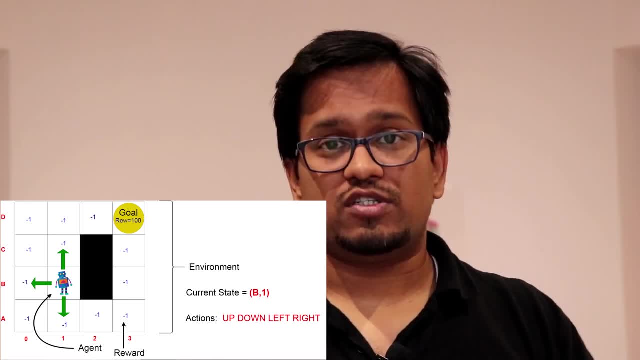 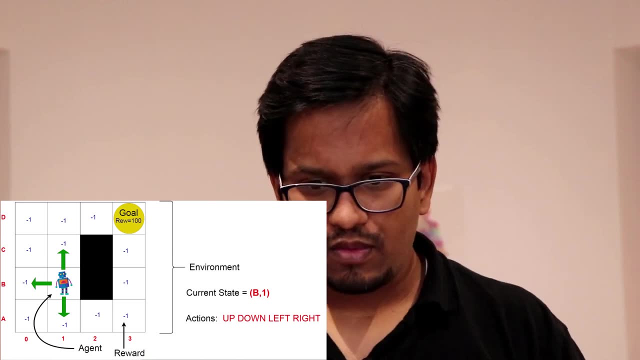 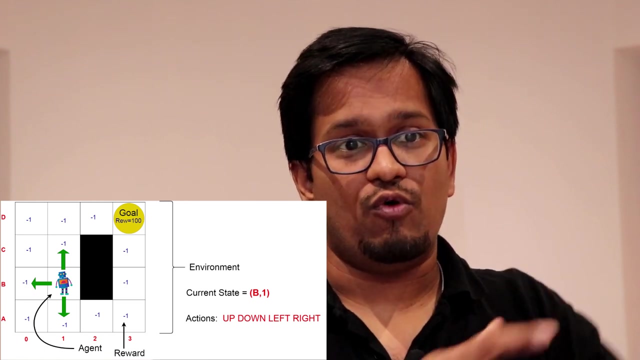 what reward i am going to, what total reward i am going to have after end of the total episode or after end of a fixed number of steps. so sometimes it has, it might get a small reward in the next step, but it can be a way to get more reward in the in the upcoming states. so in the next video. 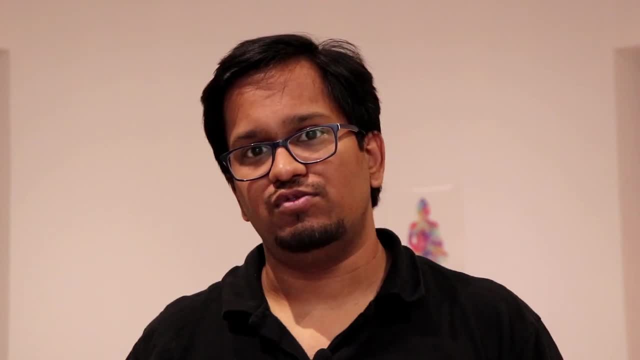 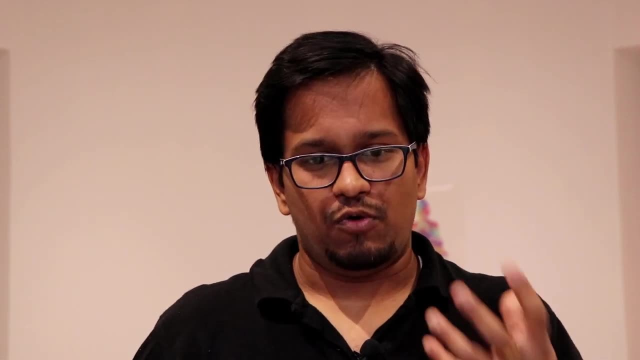 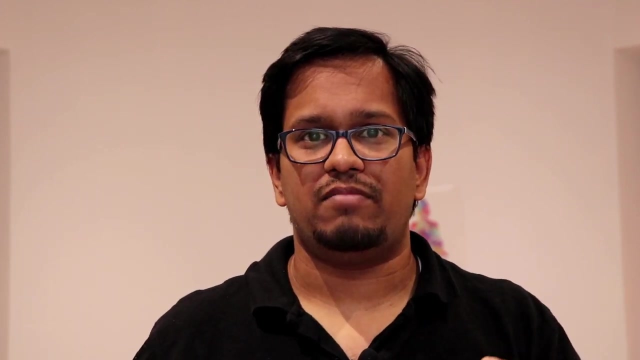 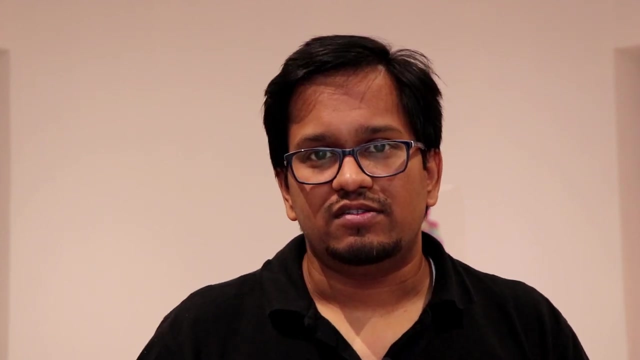 we are going to talk about mainly two algorithms to solve this problem. so solving these problems means finding a policy. so what is a policy? policy is a kind of function which defines what actions should be taken by the agent in a particular state. so we are going to find out that function. so we want to optimize that function. we want to optimize. 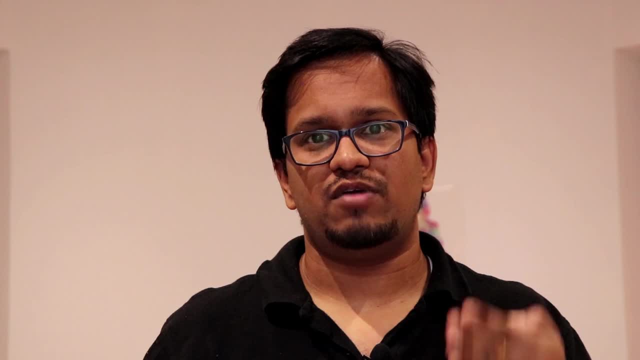 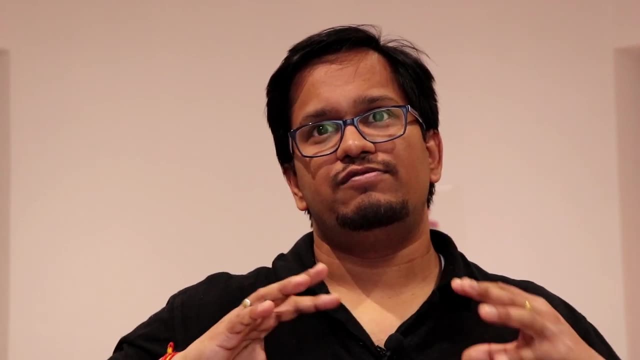 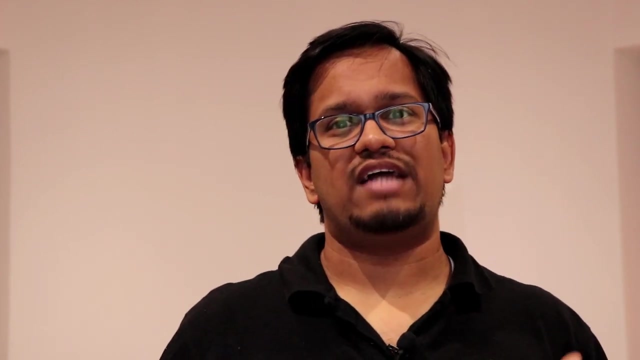 that function in such a way that the agent gets maximum reward, maximum cumulative reward- in the environment, how we can do that. so there is a very beautiful algorithms to deal with that and in the next video onwards we are going to talk about dynamic programming and using dynamic programming.